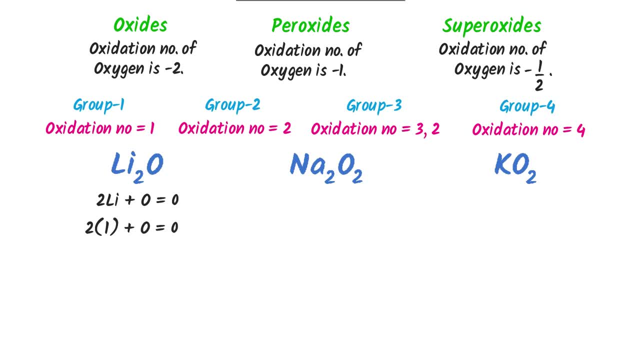 So I write 2 into 1, plus oxygen is equal to 0. I get 2 plus oxygen is equal to 0, or oxygen is equal to minus 2.. So the oxidation state of oxygen in this compound is minus 2.. Thus this: 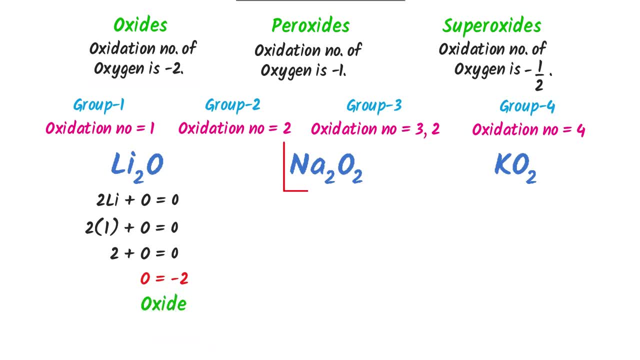 compound is oxide. Secondly, in this compound there are 2 atoms of sodium and there are also 2 atoms of oxygen. I write 2 sodium and there are also 2 atoms of oxygen. I write 2 sodium and there are also 2 oxygen and there are also 2. oxygen is equal to 0. We know that the oxidation 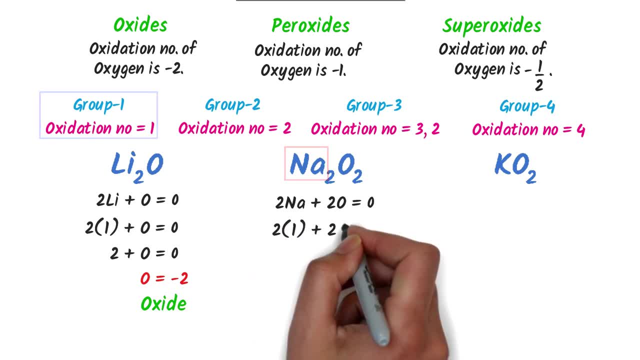 state of sodium is 1.. I write 2 into 1 plus 2, oxygen is equal to 0. or 2 plus 2, oxygen is equal to 0. or oxygen is equal to minus 2 divided by 2.. I get oxygen is equal to negative 1.. 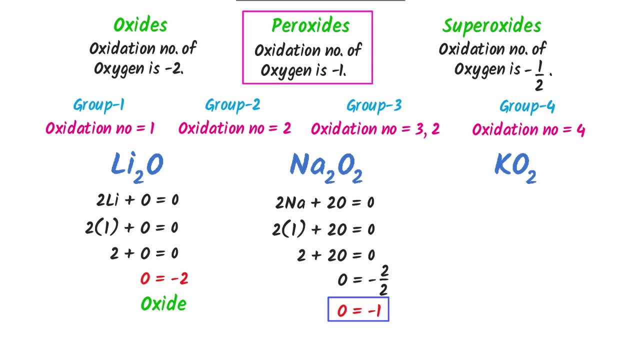 Thus this compound is peroxide 39.. Thirdly, in this compound there is one atom of potassium and there are two atoms of oxygen. I write: potassium plus two oxygen is equal to zero. The oxidation state of potassium is: one plus two. oxygen is equal to zero. 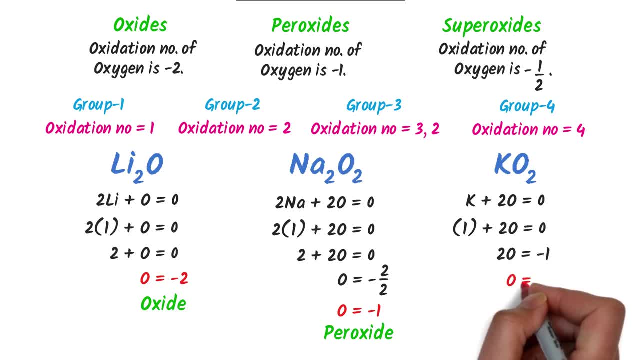 Our two oxygen is equal to negative one. our oxygen is equal to negative one divided by two. Here, in this compound, the oxidation state of oxygen is negative one, thus it is superoxide. Thus, using this trick, we can easily find oxides, peroxides and superoxides. 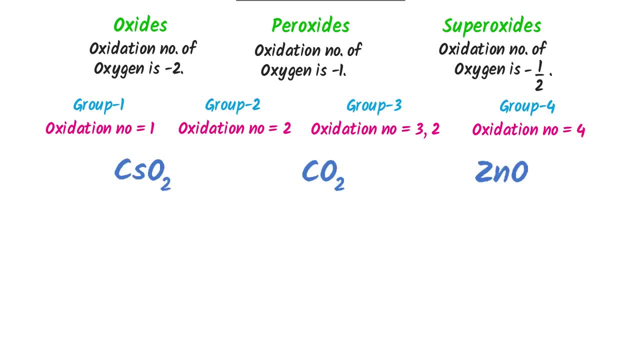 Now let me teach you medium level question: Find the oxidation state of the following compounds. Well, I write cesium plus two, oxygen is equal to zero. We know that the oxidation state of cesium is positive. So I write: one plus two, oxygen is equal to zero. 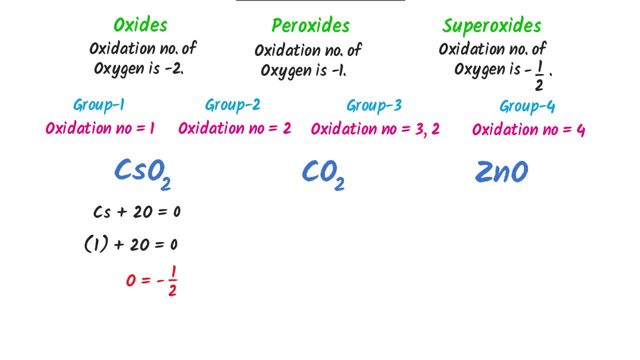 After calculation I get: oxygen is equal to negative. one divided by two, The oxidation state of oxygen is negative. one upon two. So this is superoxide. Secondly, I write: carbon plus two, oxygen is equal to zero. We know that the oxidation state of carbon is positive for.